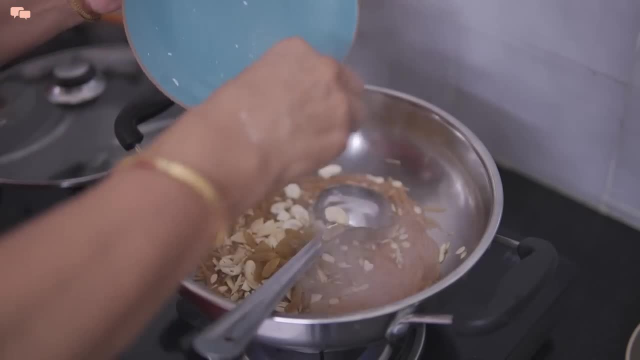 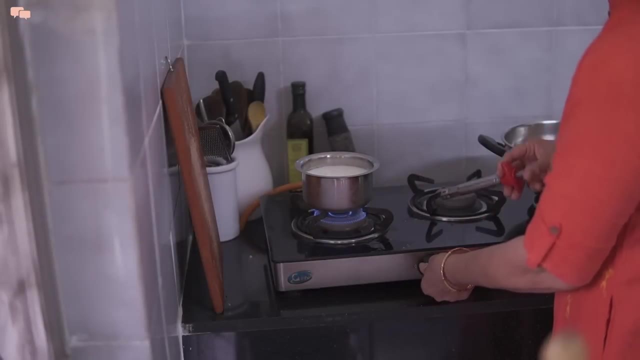 much as you can give to your child. Add the rest to the kheer Now. while the nuts and semiya soften, boil another 1 litre of milk separately, saving for as much as you can give to your child. Then add all the other ingredients to the kheer. 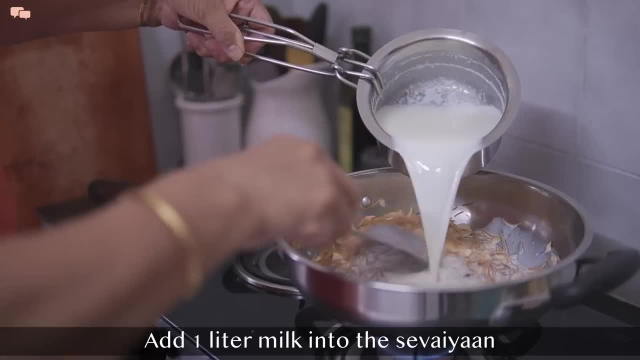 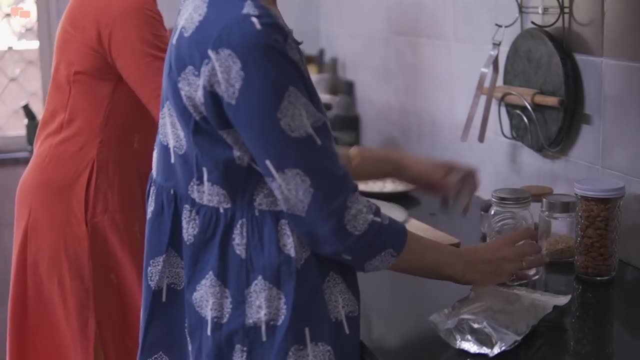 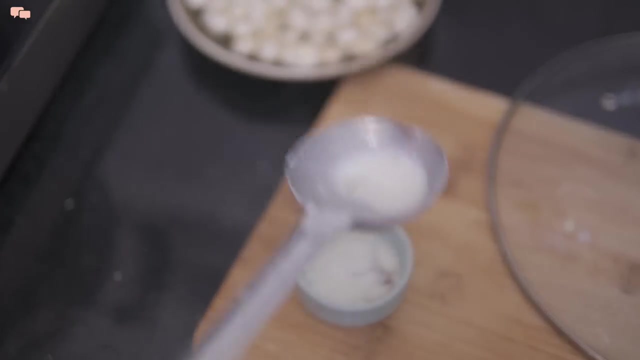 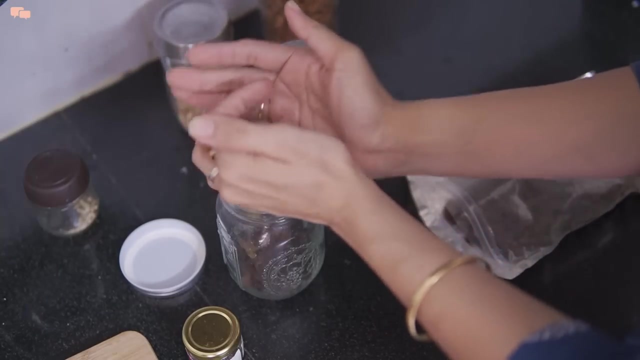 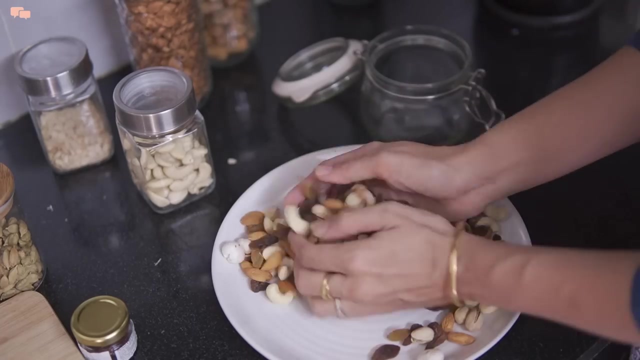 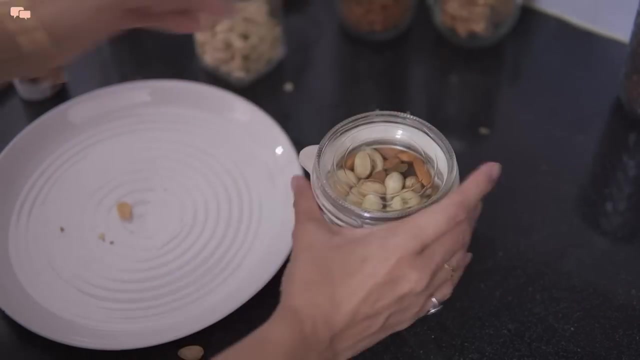 before adding to the semia mix, Feel free to add richness and fragrance of kesar into the kheer And keep stirring it till milk starts boiling. Dry fruits in my house usually go unattended when not inside, So I will make a quick trail mix to keep at my snack bar as another quick snack for all of us. 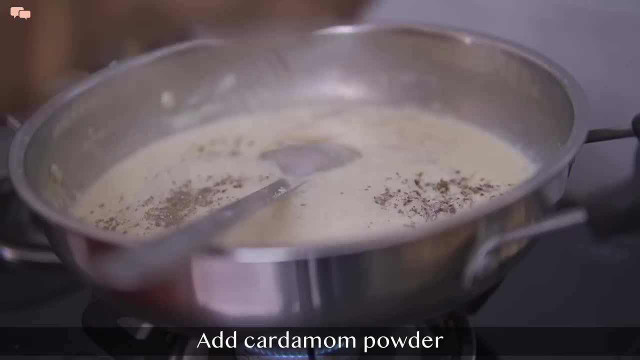 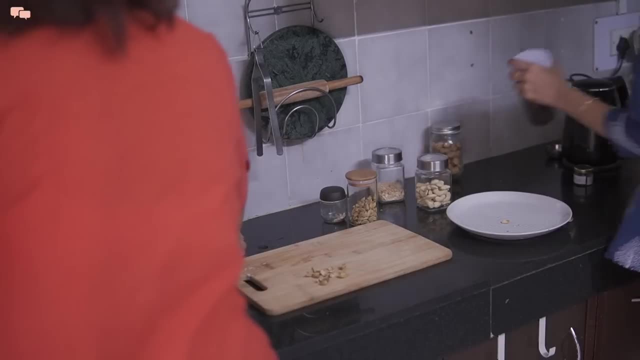 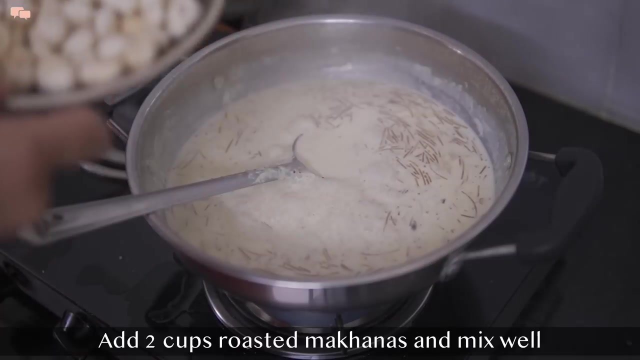 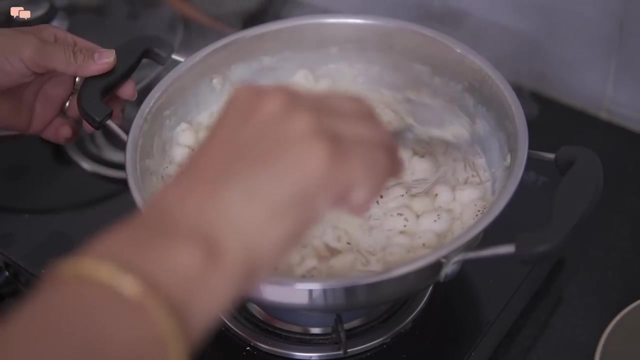 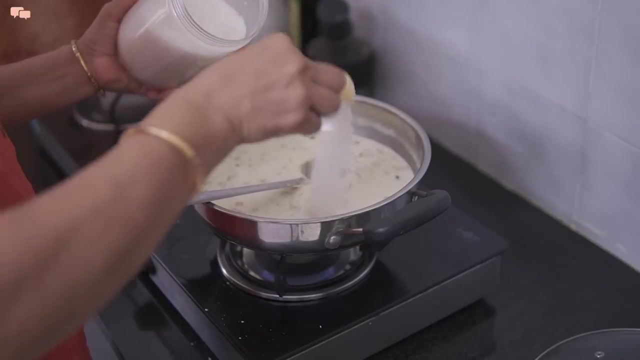 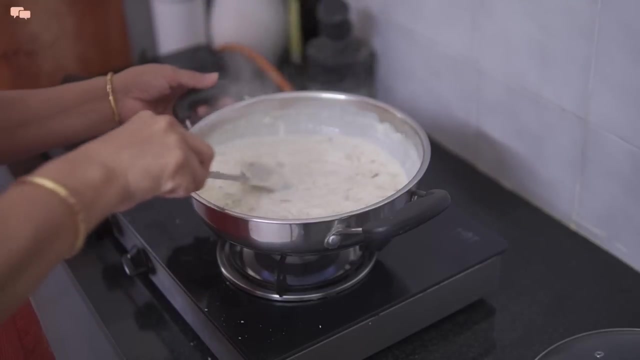 Add crushed cardamom into the kheer for the divine fragrance. Once kheer starts boiling, add the roasted makhana and mix well. For sweetness, mom is adding sugar, but if you wish to avoid it, feel free to add dates puree or jaggery, but only after shutting the stove. 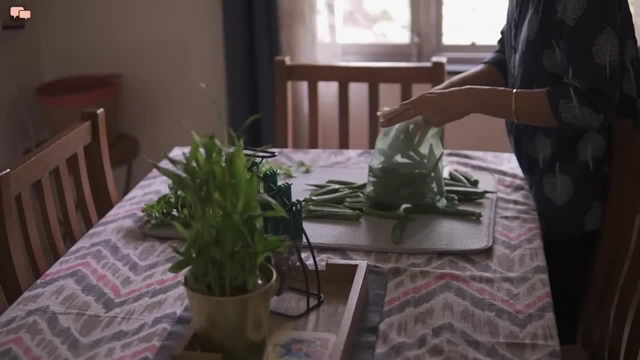 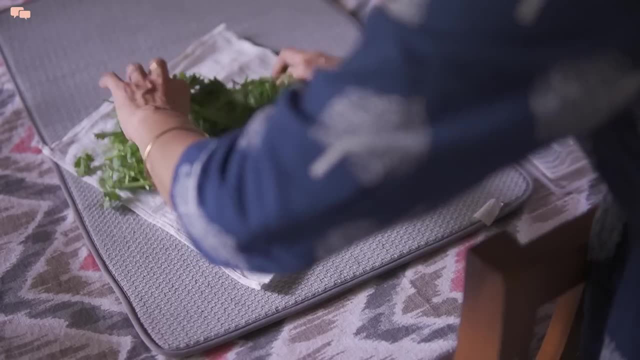 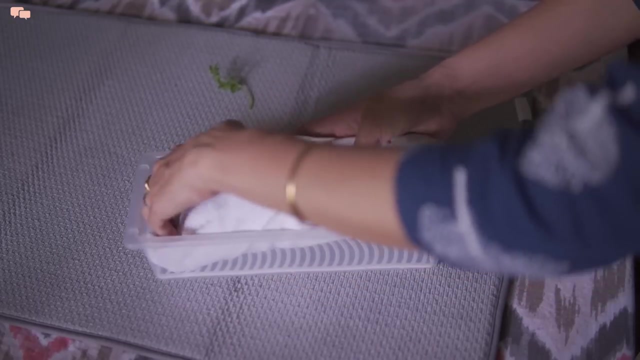 With two young kids around, I miss no opportunity to seek help, Because with extra help not only does productivity increases, but we can also meet the other demands of homemaking. to feel less burdened, I am thankful that mom was here and we made the best of this time together. 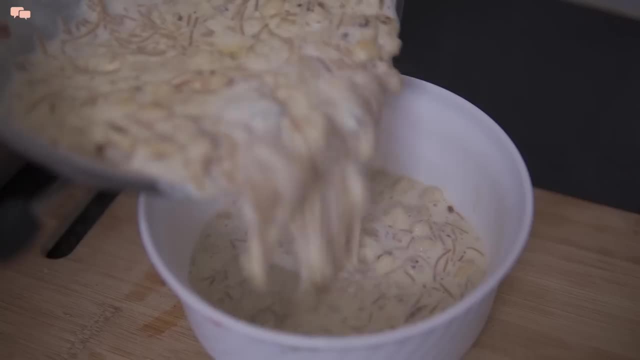 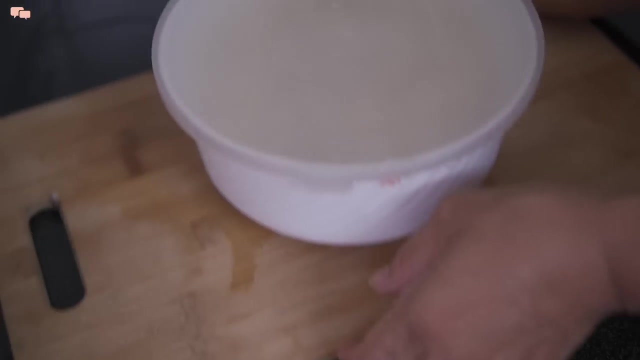 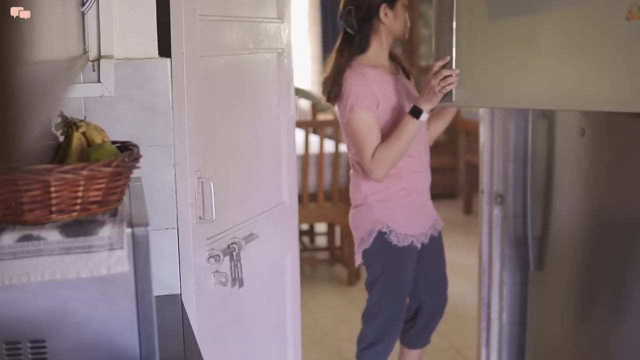 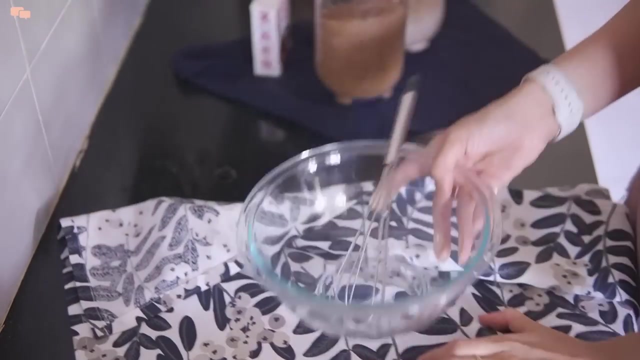 Kheer is ready, and mom was super happy to have cooked something with love for kids before leaving from here. Well, mom did her bit and I decided to continue with this task and create something that not only Ruthvi and Dhaire but Karthik also enjoys a lot, and so I decided to make some super healthy cookies. 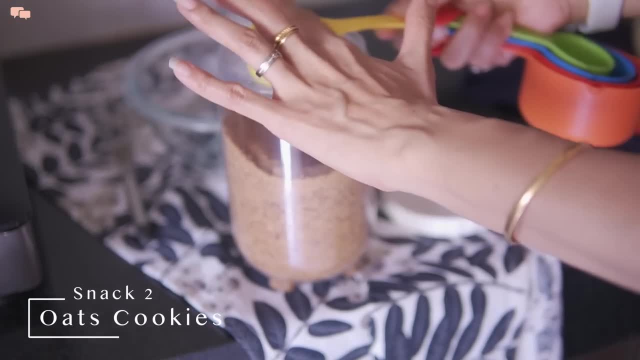 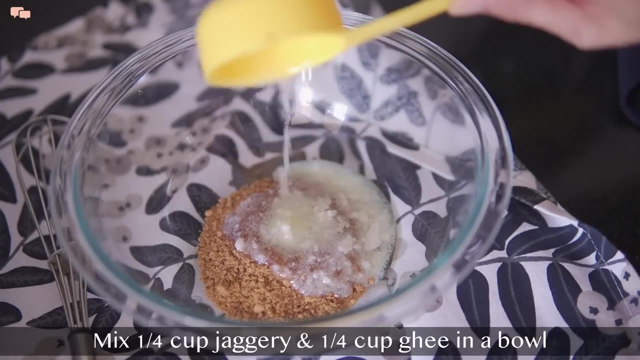 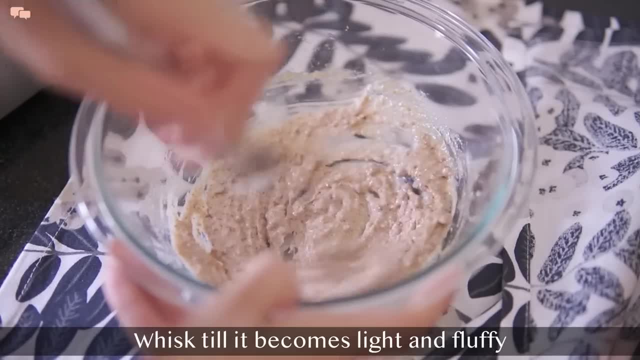 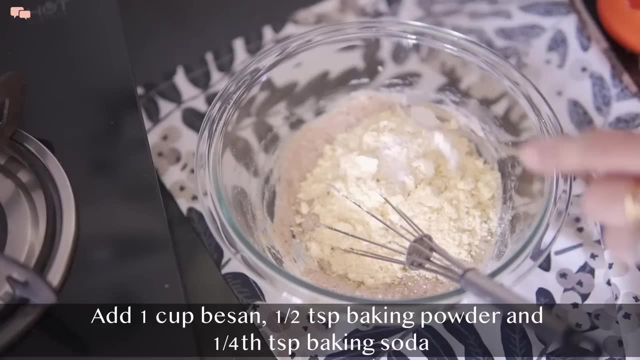 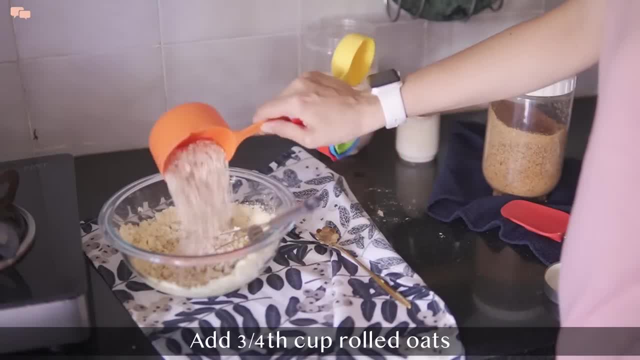 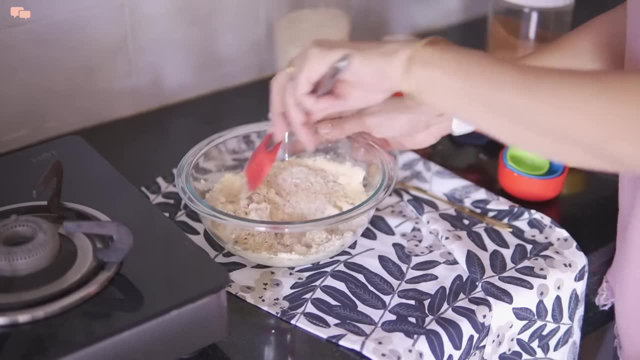 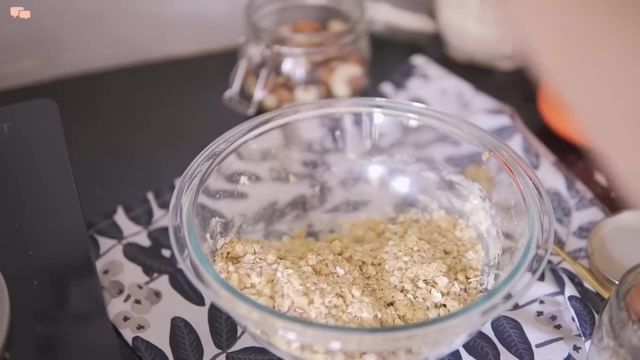 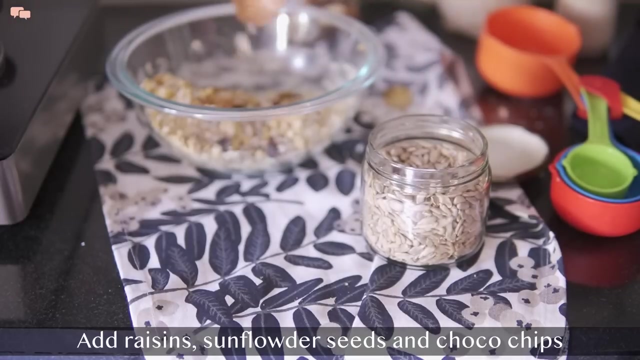 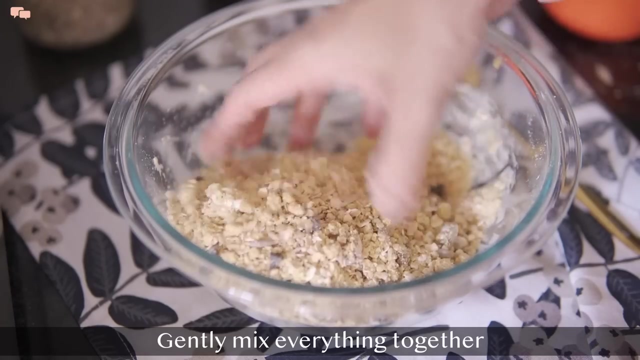 Next, in dry ingredients, I will mix 3.4 cup of rolled oats. I do not miss a chance to sneak nuts and seeds into kids diet, so in goes some raisins, sunflower seeds and chocolate chips for the fun element. Now I'll gently mix everything together. 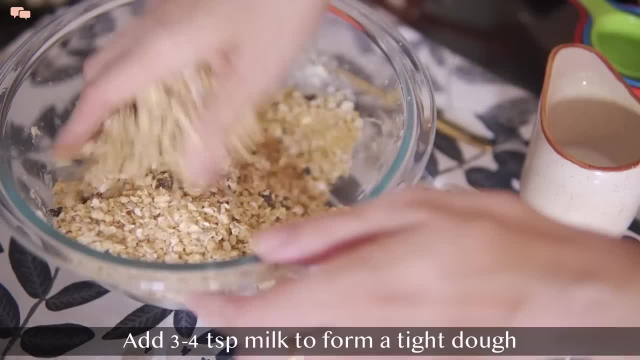 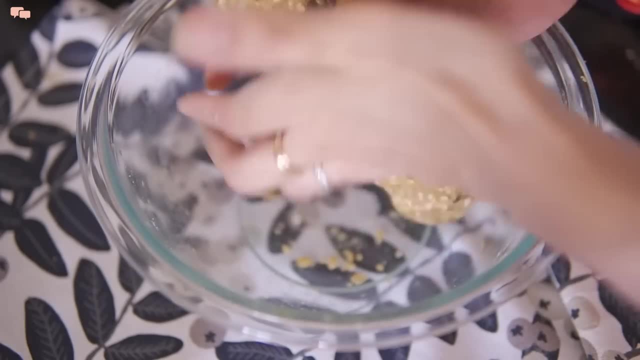 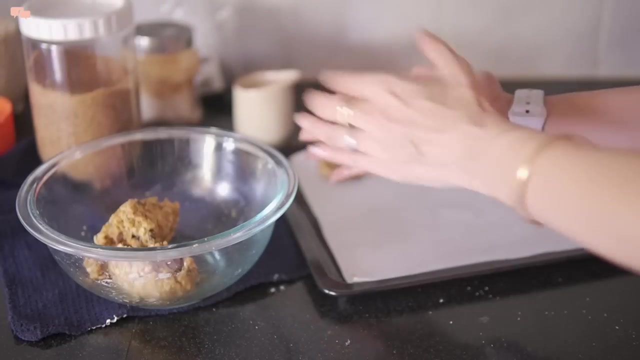 In the end, to bind the mixture, I'll add 3-4 tsp milk till it forms a rough, tight dough. I'll bake it in the oven at 175 degrees for 20 minutes, as it takes less time in the oven, but you can bake it in a kadai for 30 minutes or so. 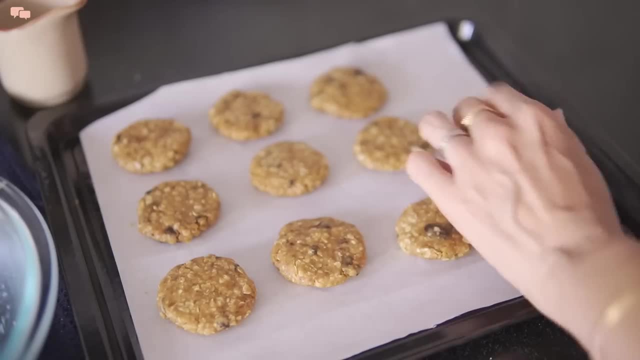 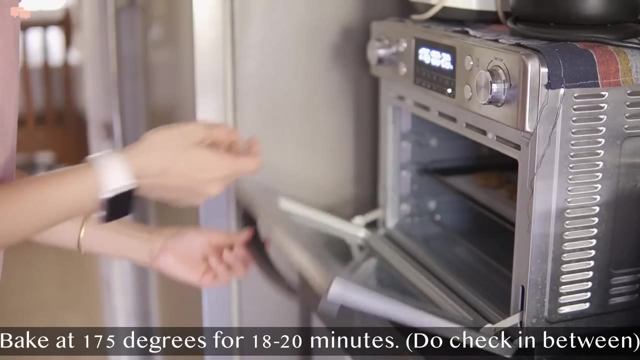 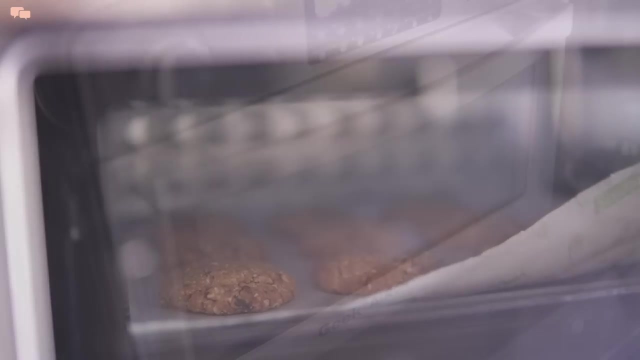 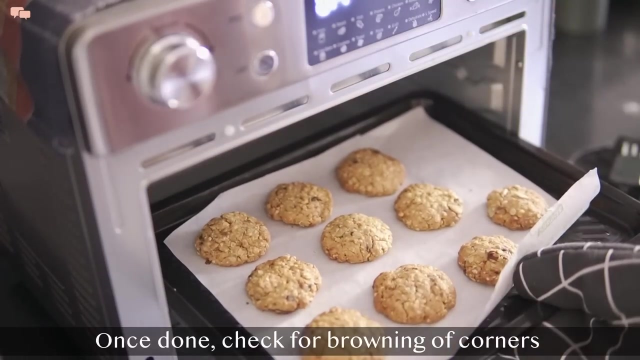 Keep checking in. between, This much dough will make some 10 cookies and while I'm forming the shape, I've kept the oven for pre-heating. After 20 minutes, I'll check for the edges if they have turned brown, as this is the indication. 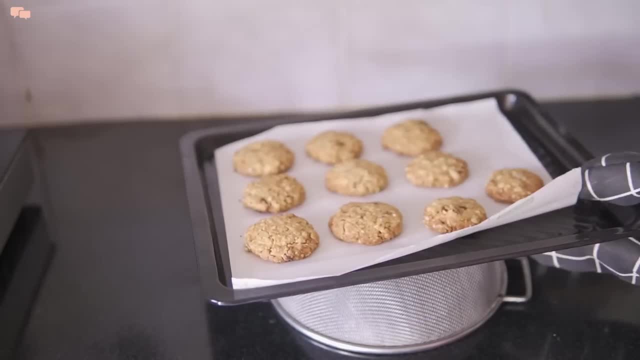 that the cookies are done, and now I'll keep it outside to cool down a bit. Now I'll check for the edges if they have turned brown, as this is the indication that the cookies are done. and now I'll keep it outside to cool down a bit. 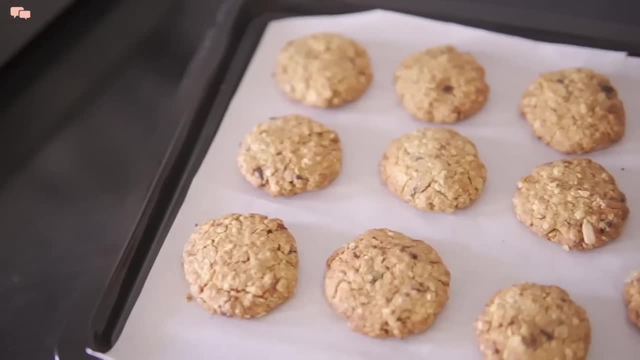 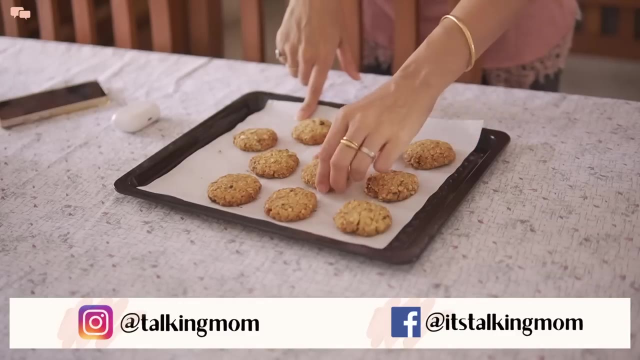 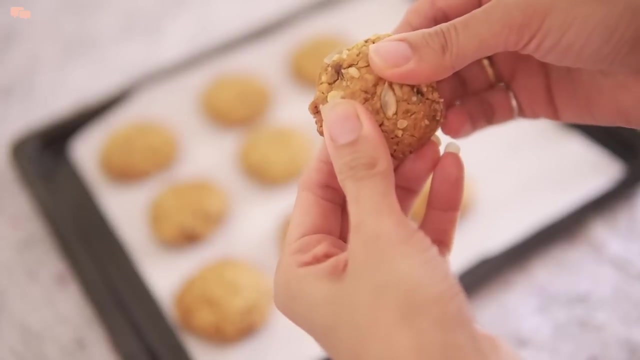 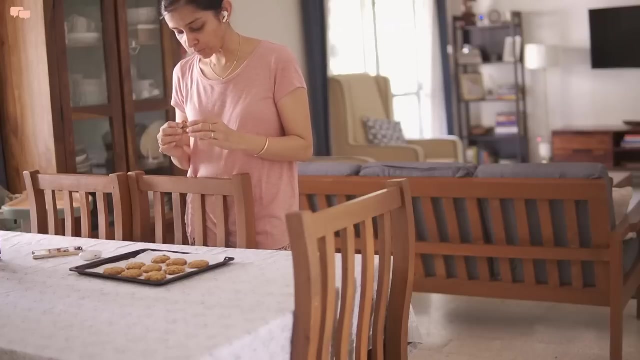 Once they cool down, remove them from the sheet and look how perfectly they are baked. They have just the right amount of crunch to them and look absolutely cafe like. Healthy homemade cookies are so satisfying. Do make them, as they make a great snack for kids- in tiffin boxes too. 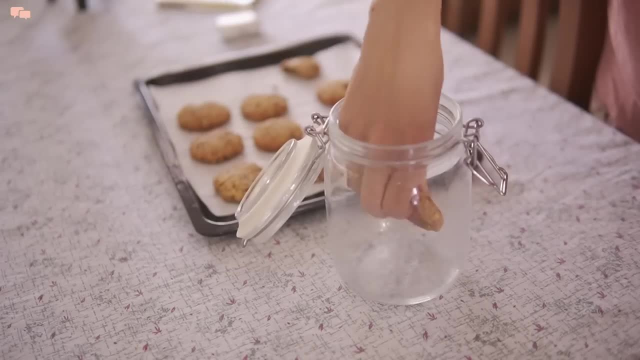 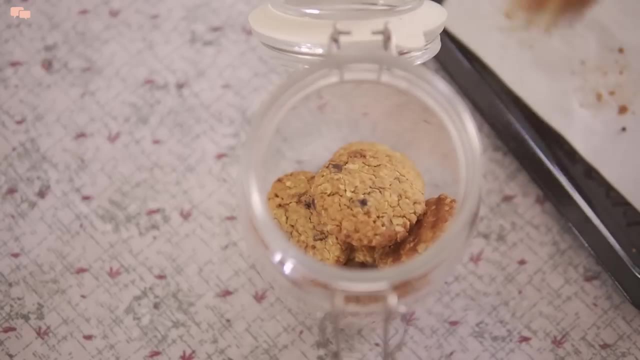 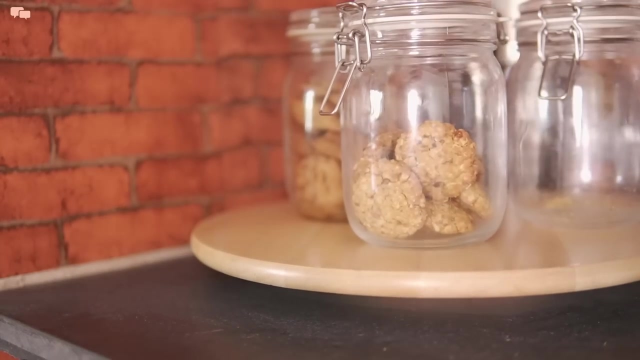 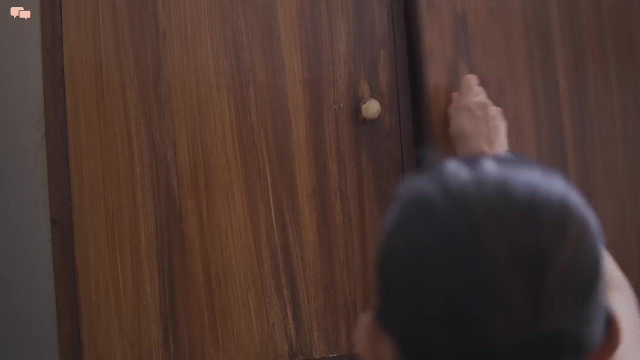 I'll see you in the next video And let me know in the comments how they actually turned out. In the afternoon, after the kids had slept, with the minimum time available, I decided to get two quick snacks ready. First one is puffed rice bars. 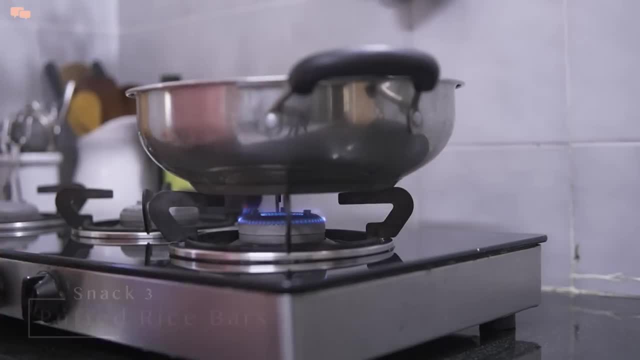 And it literally takes just a few minutes to get ready. And it literally takes just a few minutes to get ready. And it literally takes just a few minutes to get ready, And for that I'll first dry roast some puffed rice in a kadhai to take all the. 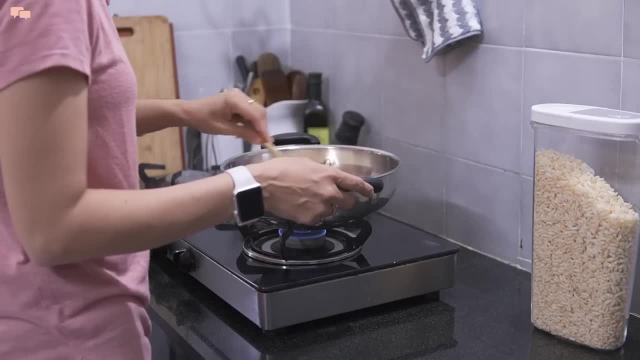 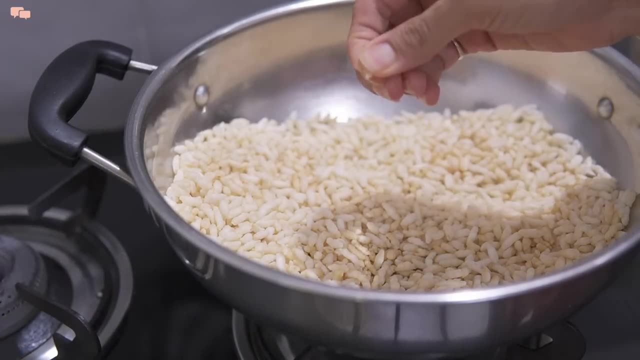 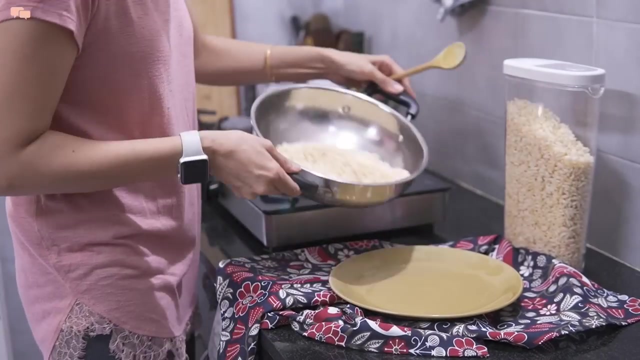 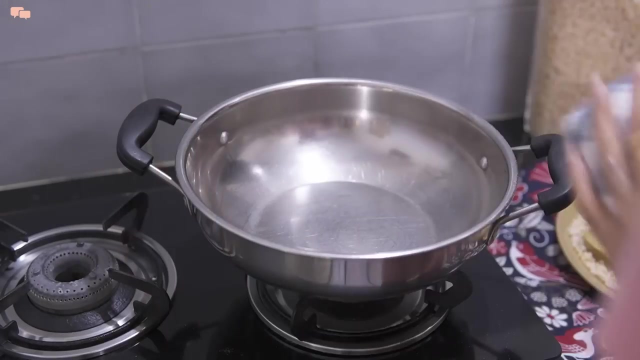 moisture out. It's not a new recipe, but this one is a kids delight and gets ready so quickly. Once done, I'll cut them into small cubes. Once done, in the same kadai I'll add 2 tsp ghee and 1 cup jaggery. 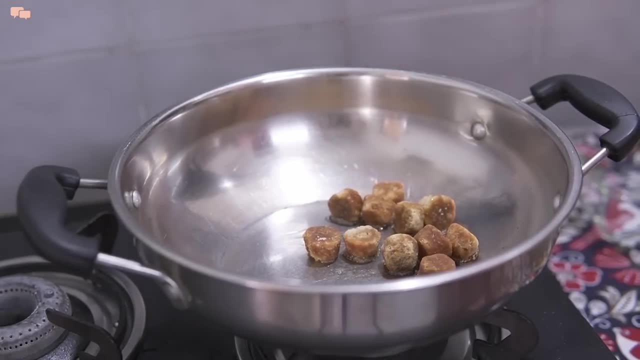 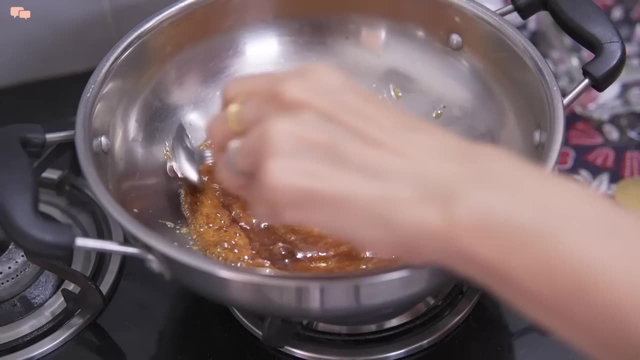 Ghee is basically to avoid jaggery from sticking at the bottom of the pan While jaggery melts. I'll coat this baking sheet with some ghee. It takes 3-4 minutes for jaggery to melt, and do the water test till you get a soft ball. 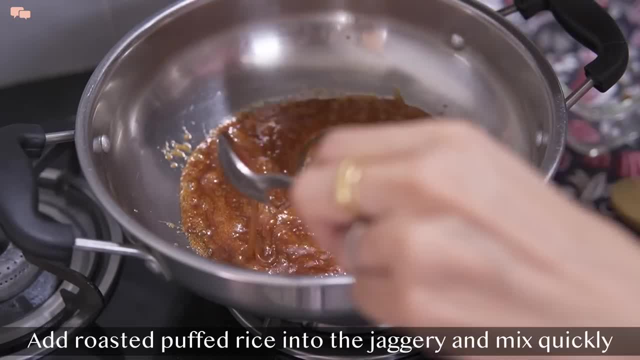 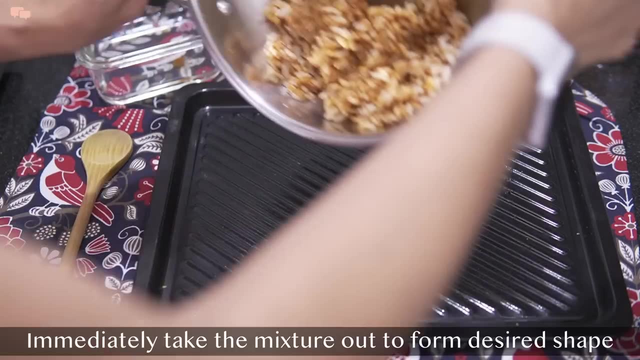 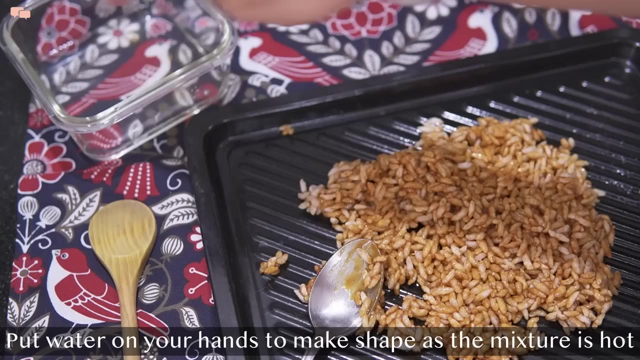 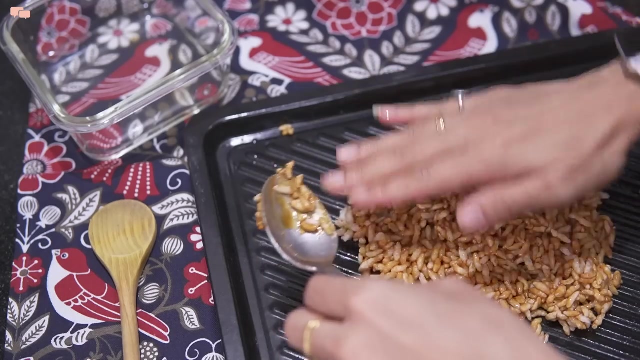 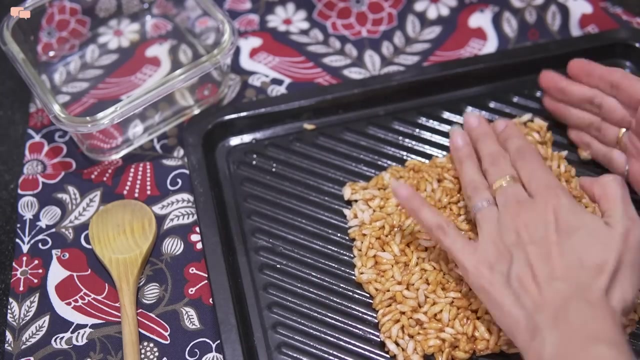 consistency. Switch off the flame and add the puffed rice into the pan. Give everything a quick toss and transfer it into the sheet. With the help of water, I'll spread the mixture to form a square shape. I am doing a makeshift arrangement, but if you have a square cake tin, go for it. 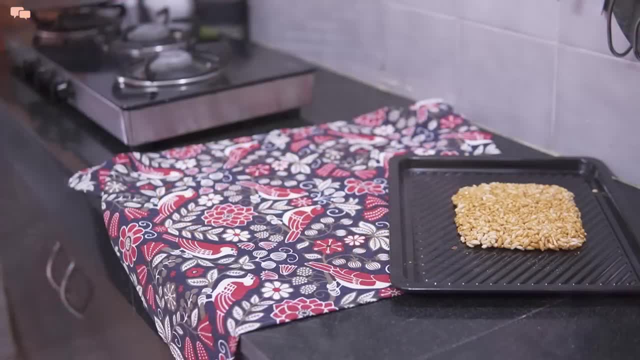 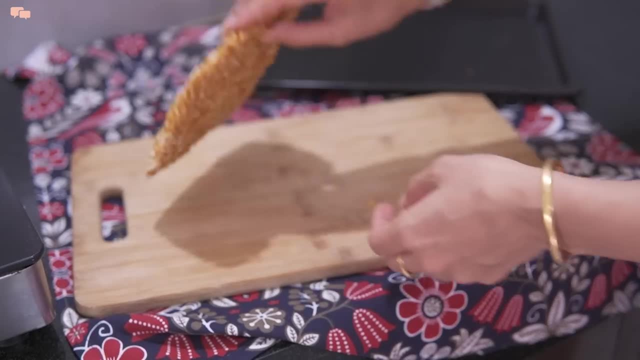 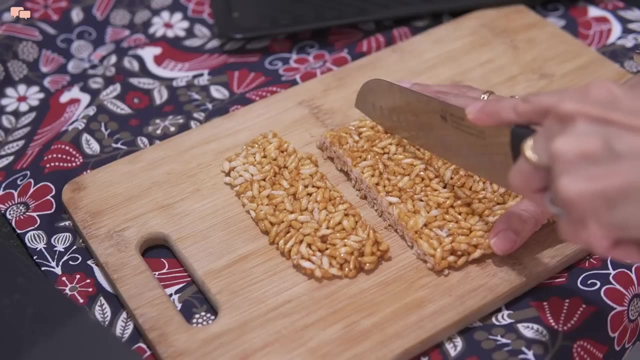 The mixture will set within 5 minutes. Now I'll add the jaggery. Now take this block and cut them into squares. You can make laddoos as per your preference, but I find squares easier to store and well portioned bars are easier for dhere also to hold and eat. 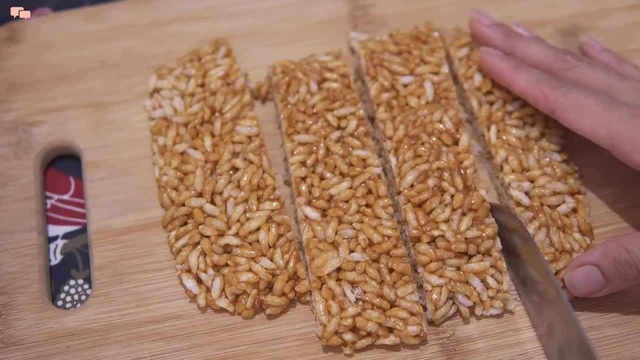 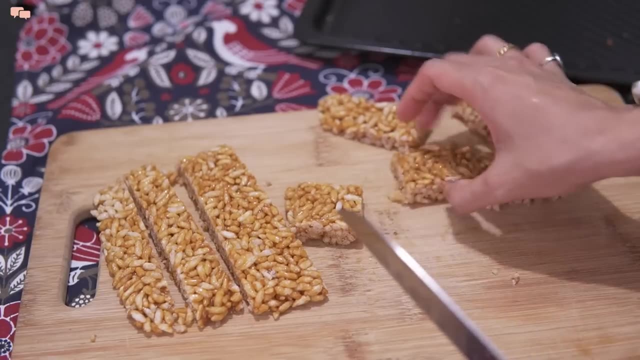 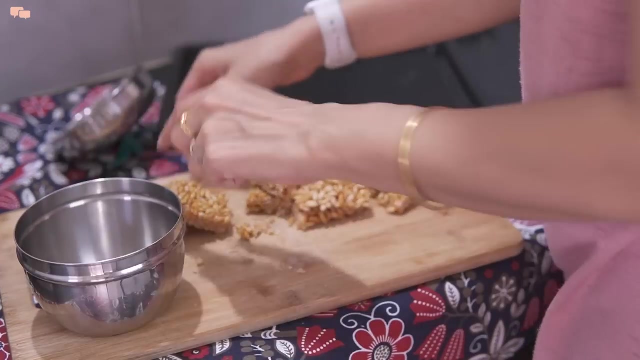 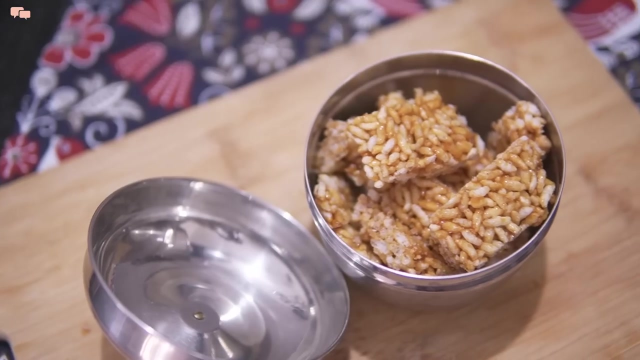 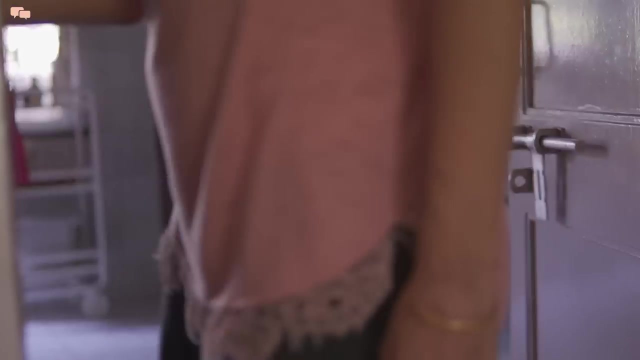 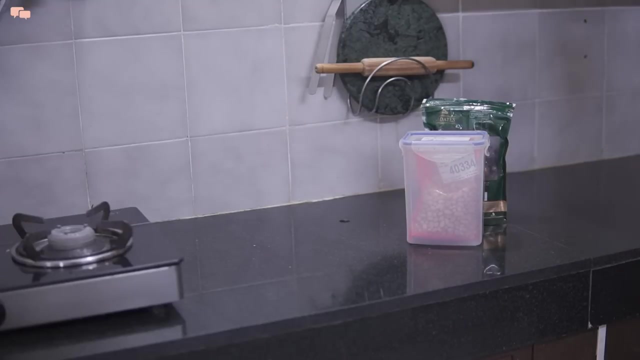 Jaggery is high in iron, and puffed rice helps boost immunity, as they are filled with antioxidants. Even I love them equally, and they are a perfect solution for my sweet cravings too. The next one takes a bit of a time, but is super healthy, and my kids love it because. 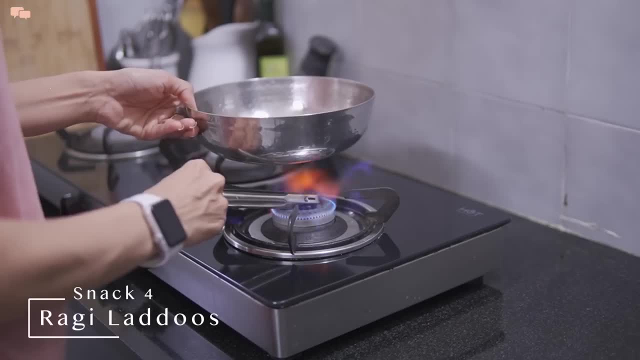 I add some kid friendly twist to this. The next one takes a bit of a time but is super healthy and my kids love it. because I add some kid friendly twist to this, I'll make ragi laddoos, or also called as nachni laddoos, and this is my take on no sugar. 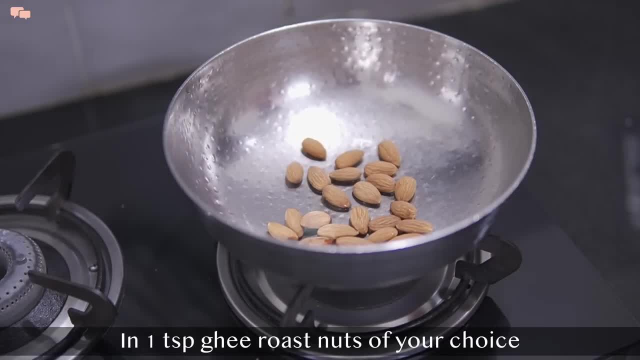 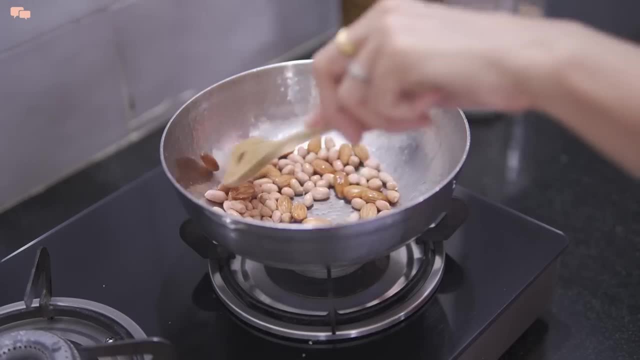 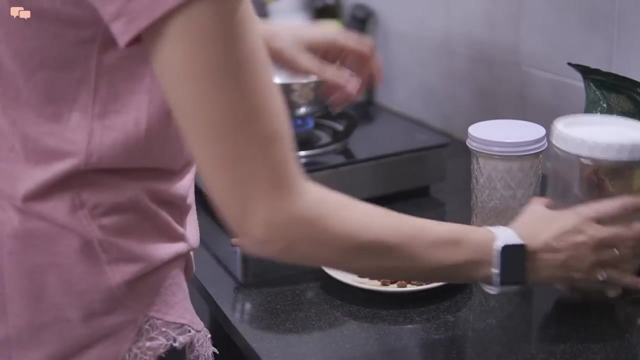 sweet laddoos. I'll first start by roasting everything, Starting by roasting some nuts in 1 tsp ghee. In nuts I'll just add almonds and peanuts. Feel free to add more if you like them. Once they turn golden brown, I'll then roast some whole oats. 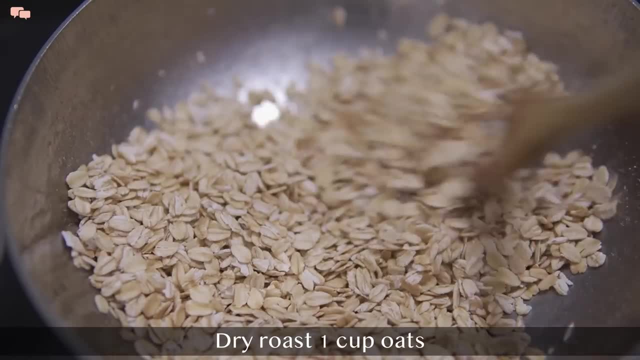 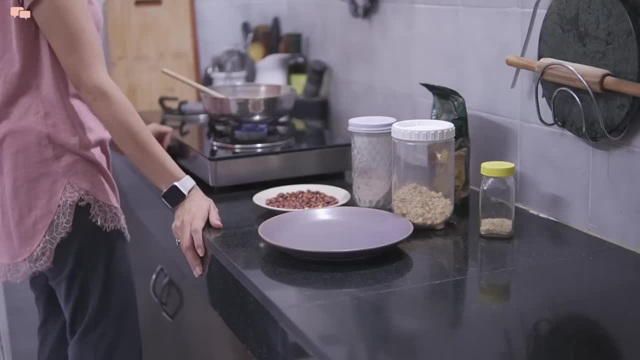 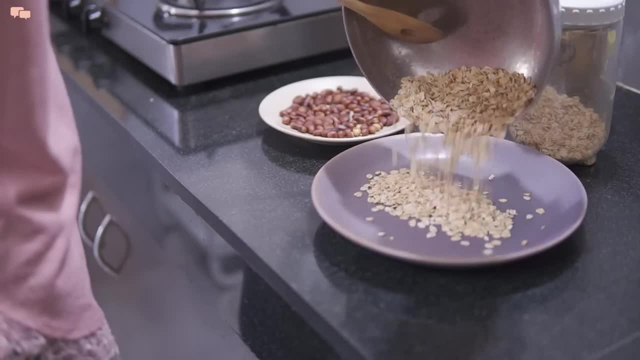 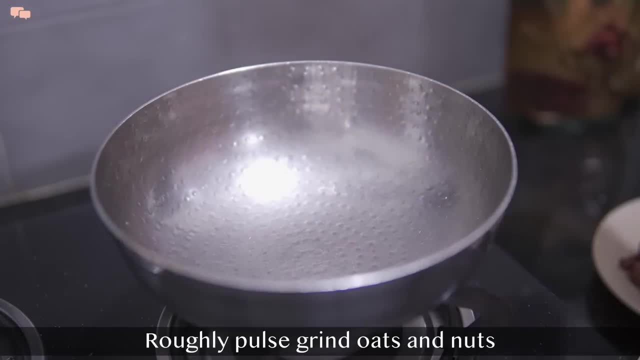 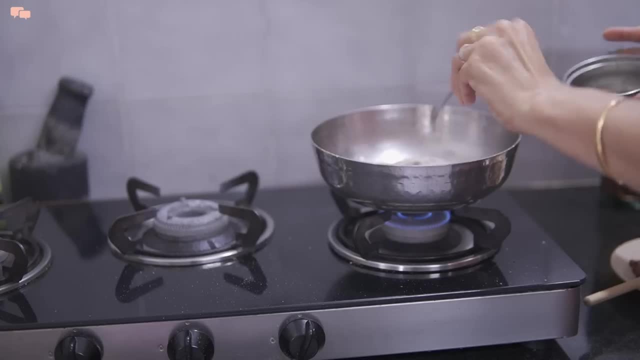 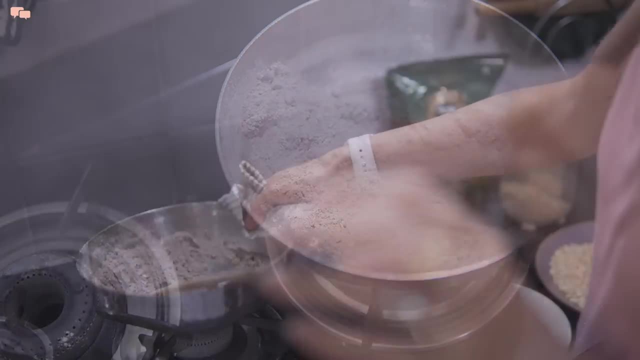 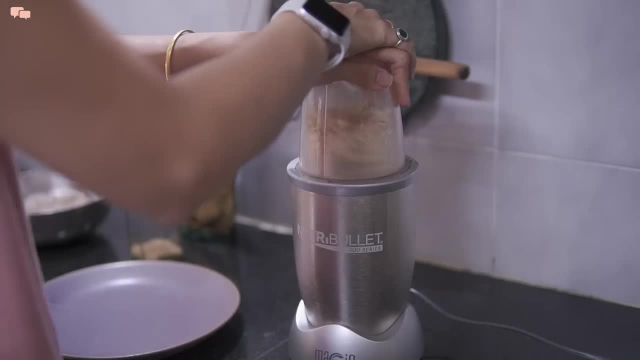 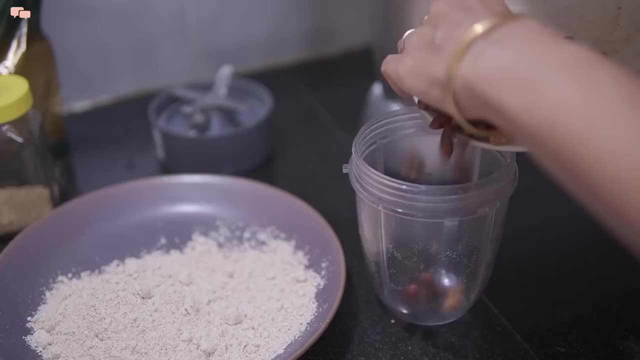 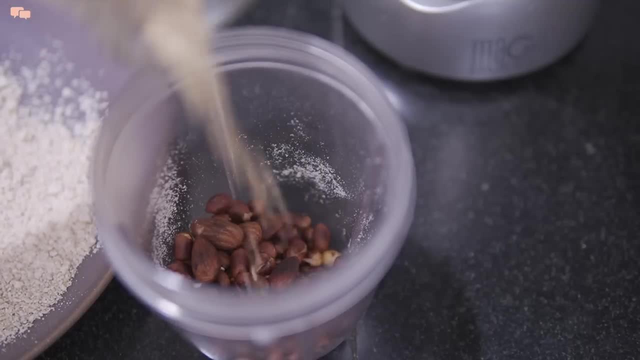 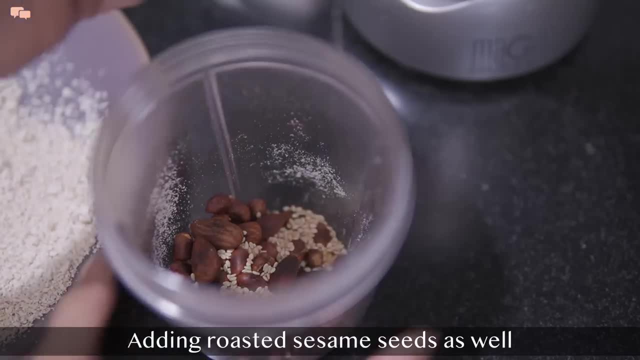 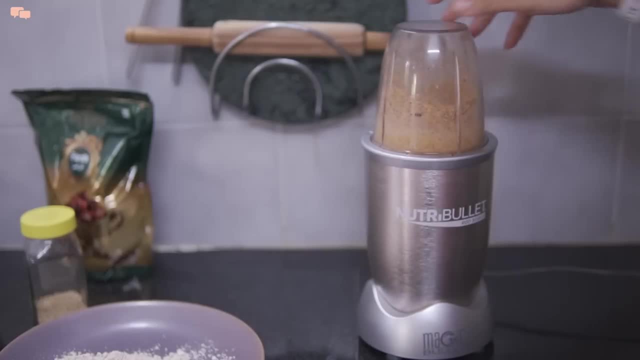 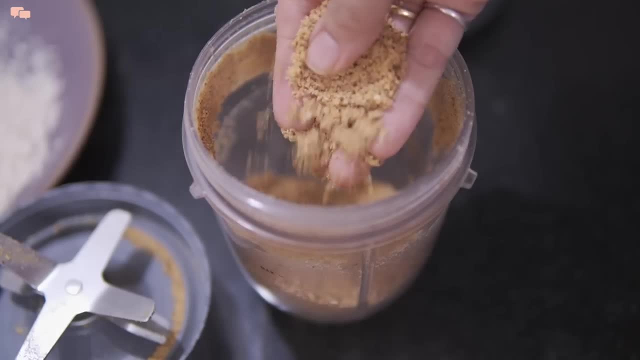 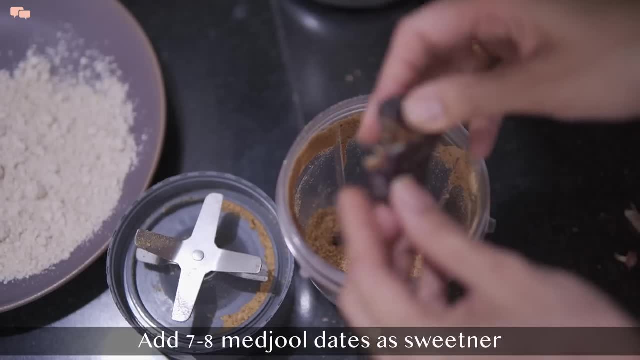 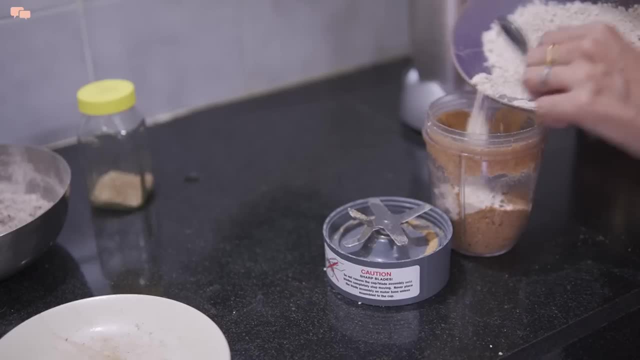 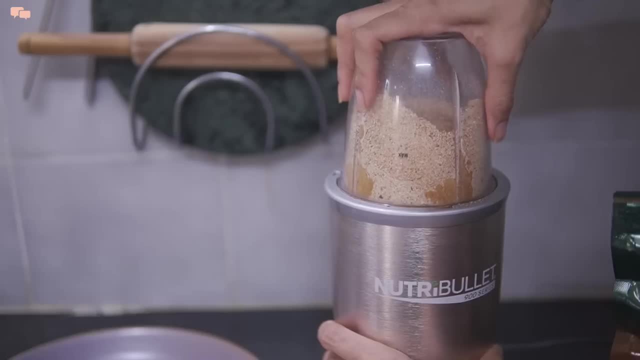 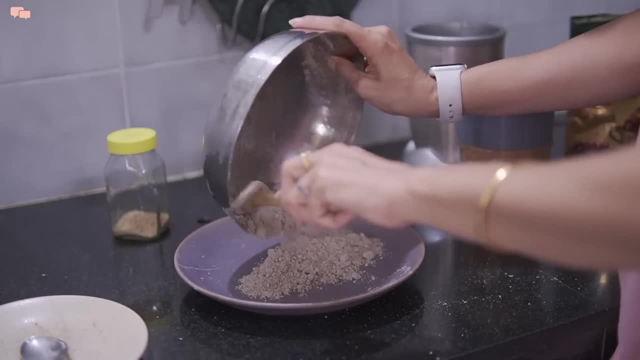 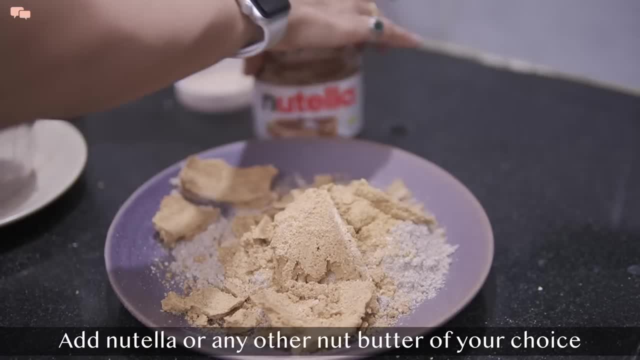 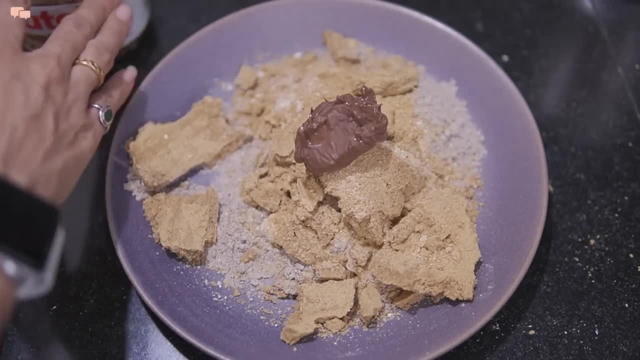 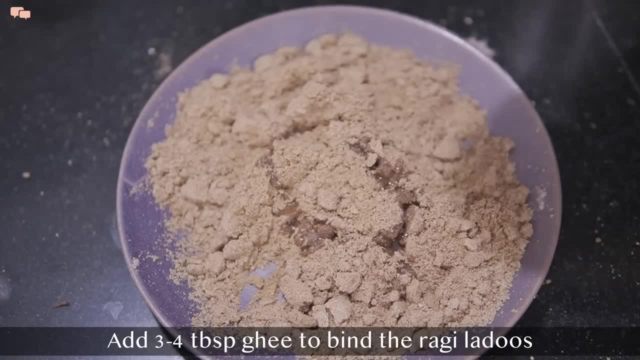 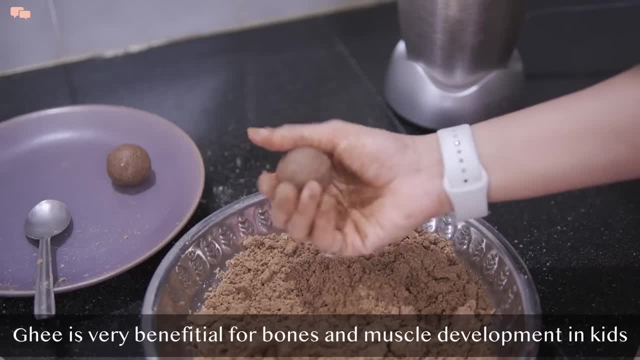 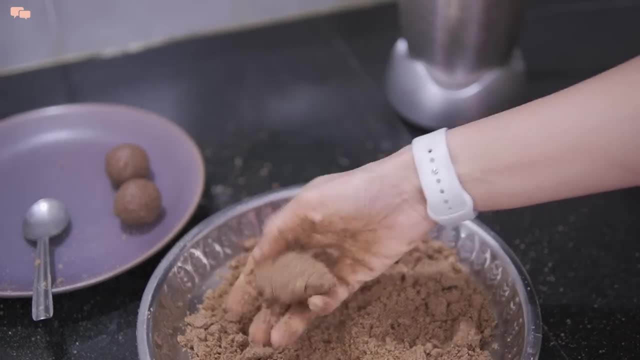 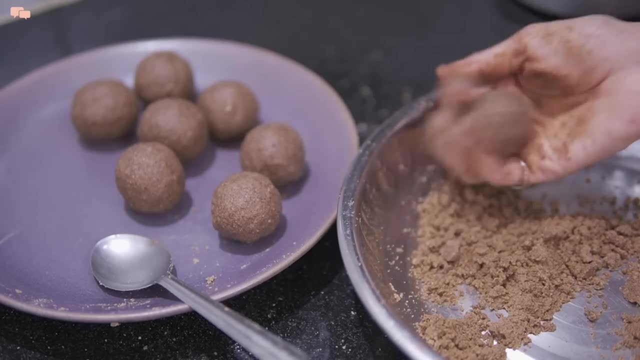 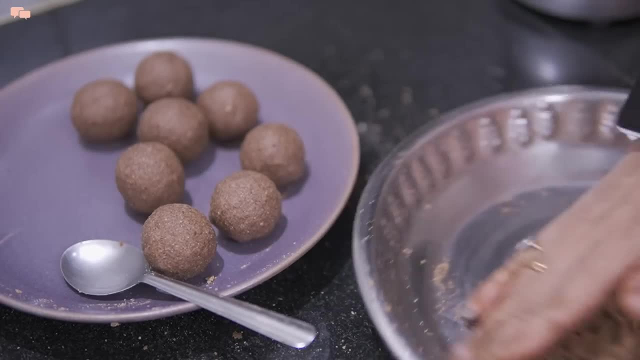 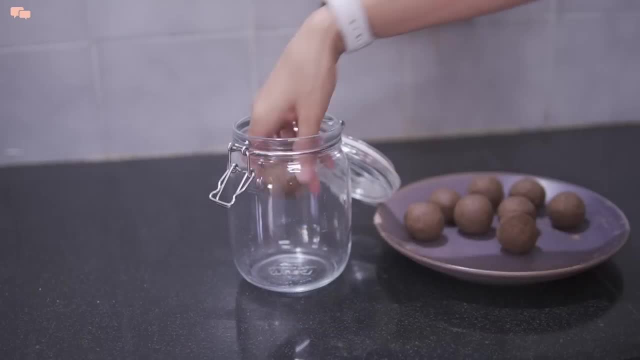 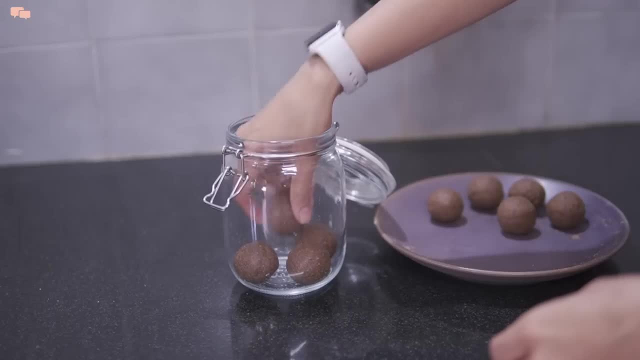 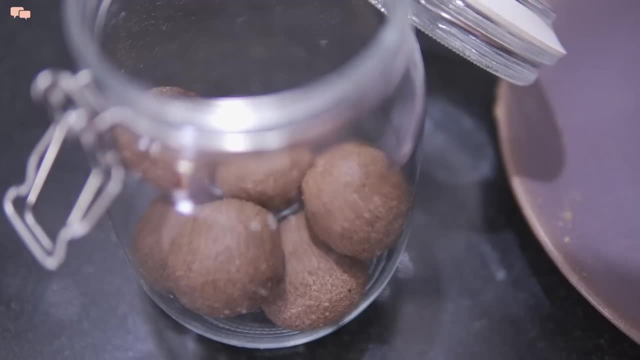